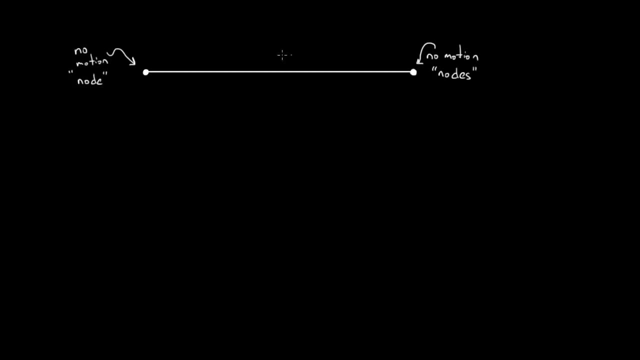 So for this string there's gonna be nodes at each end, And we'll see when you set up a standing wave. it's possible that there's nodes in the middle as well, but there don't have to be For this string, though. we're making sure. 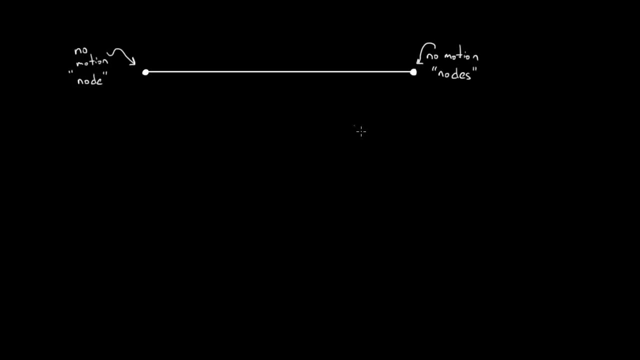 that there have to be nodes at each end. So why does a standing wave happen? and how does it happen? Well, let's say you give the end of the string here a little pluck and you cause a disturbance. That disturbance is gonna move down the line. 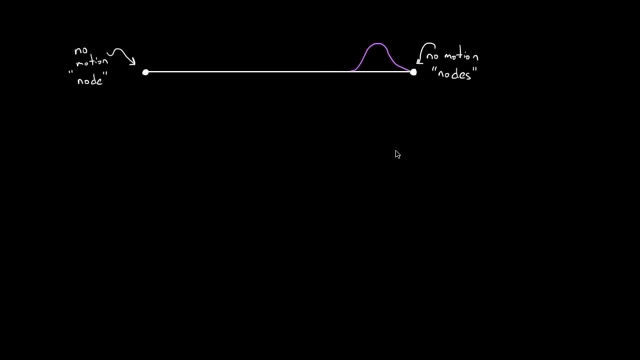 because that's what waves do. It's gonna come over here. Once it meets a boundary, it's gonna reflect back to the left. Now it turns out when a string hits a boundary where it's fixed, when it hits a node, in other words, 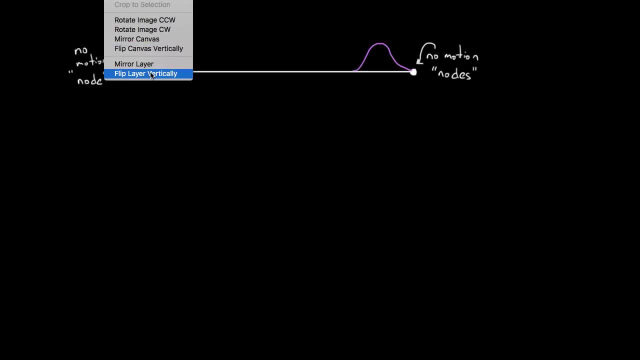 it gets flipped over. So you might have tried this before with the hose. If you send a pulse down the line, try to see how it reflects. It gets reflected upside down. That doesn't matter too much for our purposes, but every time it's gonna reflect. 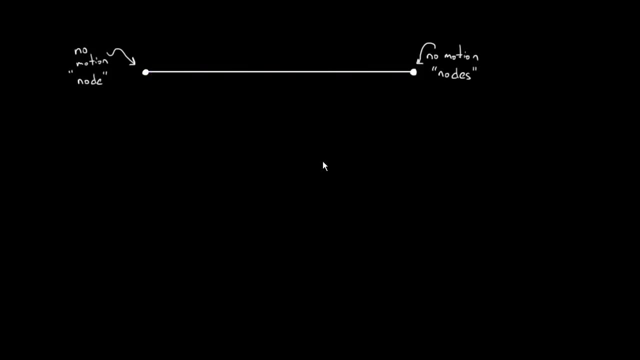 it flips its direction and it keeps bouncing. Now let's say, instead of sending in a single pulse, we send in a whole bunch of pulses. right, We send in like a simple harmonic wave. Now, when this thing reflects, it's gonna reflect back on top of itself. 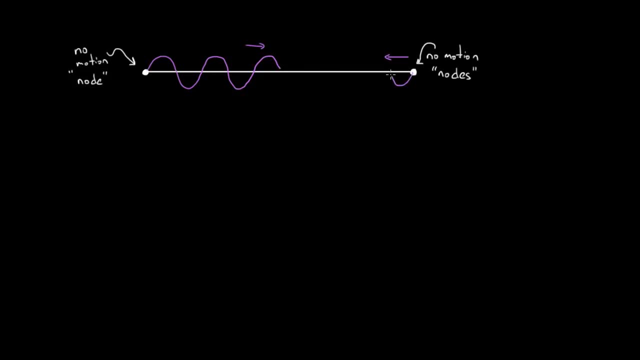 because this leading edge will get reflected upside down this way and it's gonna meet all the rest of the wave behind it and overlap with it, creating some total wave that would be composed of the wave traveling to the right plus the wave traveling to the left, 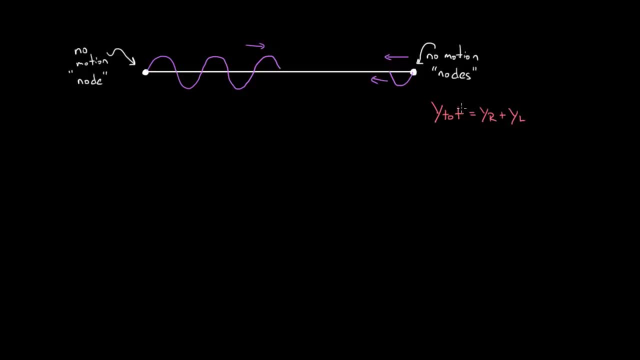 and you can use superposition and interference to figure out what that is, which for most wavelengths is just gonna be a mess. So if you just send in whatever wavelength you want and let it reflect back in on itself, the total wave you get might not really be anything special. 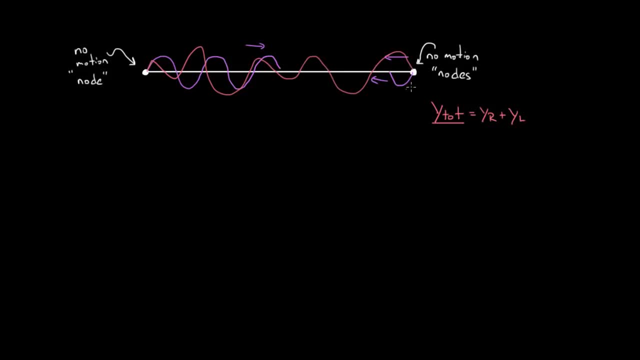 It might just be sort of a mess in here, nothing really all that interesting. However, there'll be particular wavelengths if you add up a standing wave, and I'll show you what that looks like in a minute. How do you find these special wavelengths? 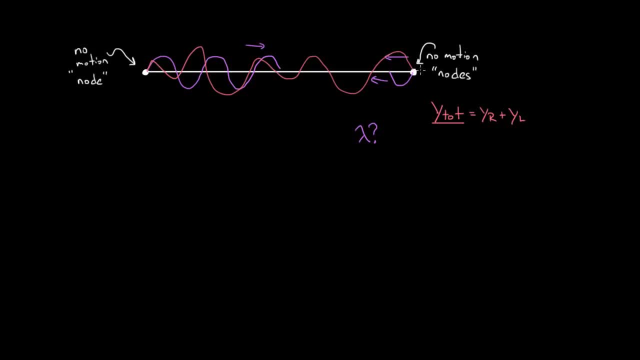 You simply ask yourself: what wavelengths could I draw on this string so that there was a node at each end? What wavelength would fit inside of this region and have a node at both ends? So instead of trying to add up a complicated superposition of waves, 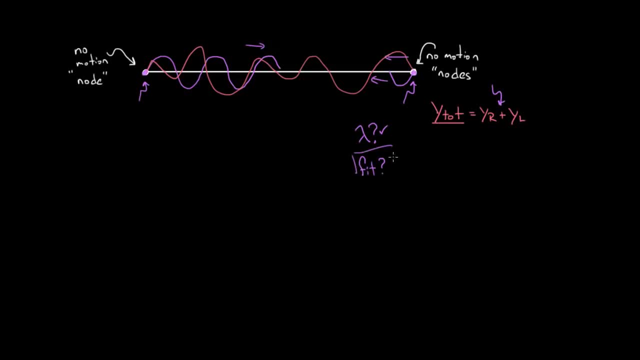 we can figure out the special wavelengths simply by drawing them and seeing which ones fit. So let's try it out, Let's get rid of all this. What wavelengths would fit in here? Well, we know what a simple, harmonic wave looks like. 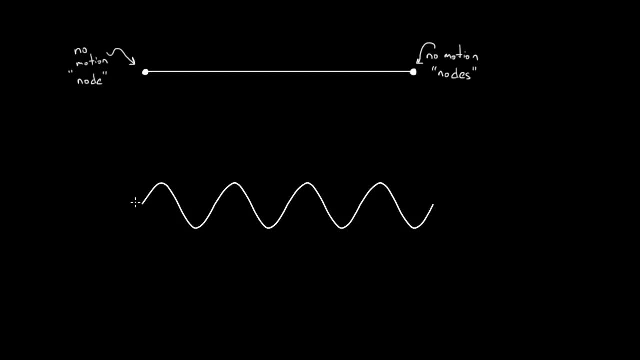 It looks something like this. So the question we need to ask is: if we start at the zero point, because I wanna make sure I have a node at the left end, what might the shape of this graph look like so that I reach a node at the other end as well? 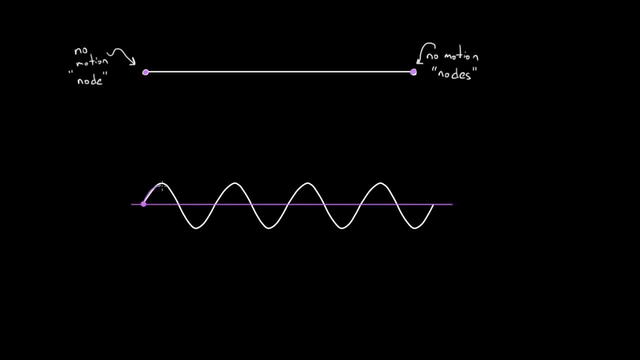 Well, the first possibility. look at it. I started a node. When do I get to a node again? I get to a node when it takes this shape. right here There's another node. So the first possibility, which is gonna be the longest, largest possibility, 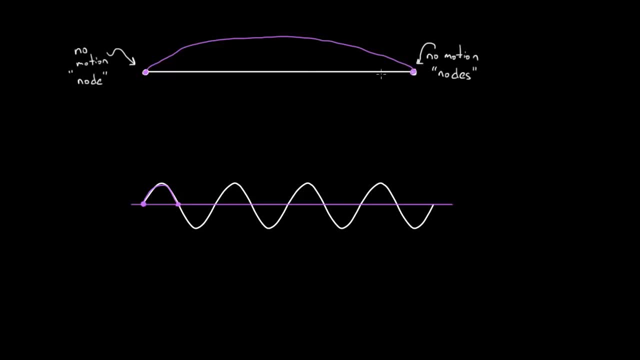 would be a wave that just kinda looked like this, Looks kinda like a jump rope. This would be the first possible standing wave you could set up on this string and that means it's special. It's called the fundamental wavelength. This is the big daddy. 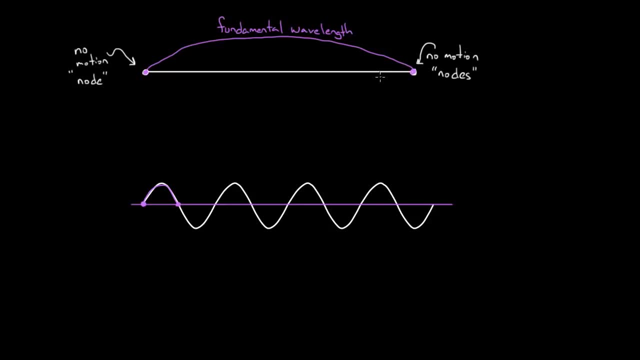 This guy dominates all the other wavelengths we're gonna meet. Yeah, there's other standing waves you can set up on here, but this one's the big alpha dog And if you let this string vibrate however it wants, it's gonna pick the fundamental wavelength. 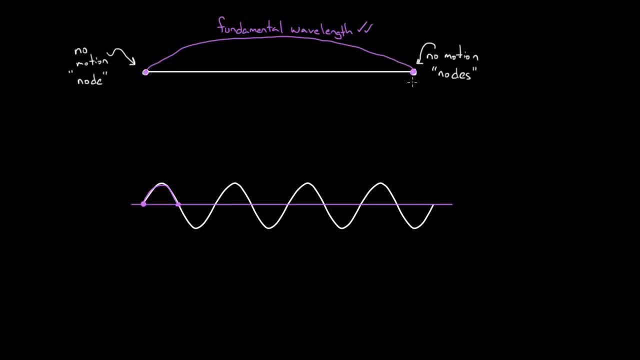 And so what would we see happen? The string's not just gonna be suspended in air like this, It's gonna be moving around, and it's called standing waves, because this peak no longer looks like it's moving right or left, This peak is just gonna move up and down. 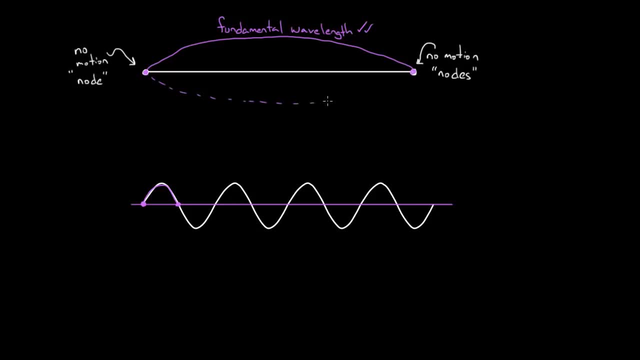 So a lot of times when we draw these standing waves we draw a dash line underneath here that mirrors the bold line, because all this peak's gonna do is go from the top to the bottom, then back to the top. It's just gonna oscillate. 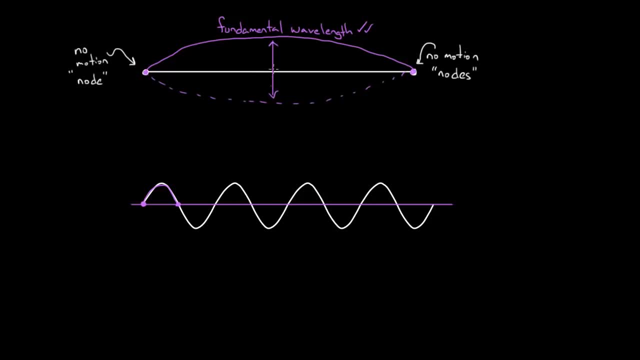 It's gonna look like a jump rope, but it's not revolving, It's just moving up then down, then up then down. It takes this shape, Then it would be flat. Then it might look something like this, And then it comes down to here: 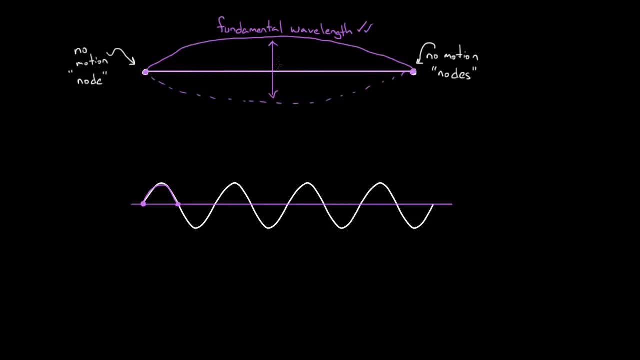 Then it goes back up and it keeps going up and down. We call it standing. It's more like dancing, It's kind of like a dancing wave, but we call them standing waves because these peaks don't move right or left. So that's the fundamental wavelength. 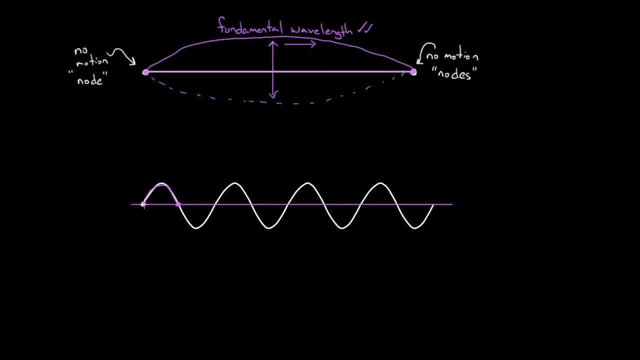 What would the next possibility look like? Let's see, We gotta go from a node. We know we have to go from node all the way to another node. That was the first one, So let's just keep going and go to the next one. 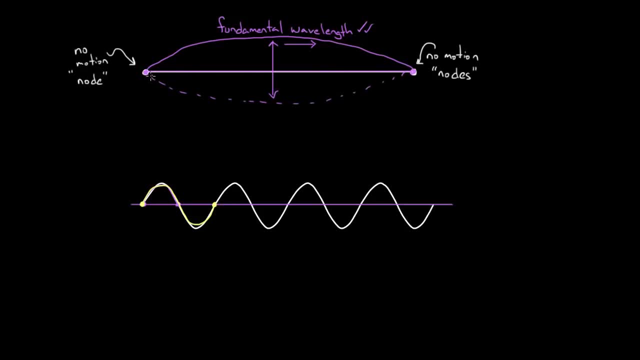 That would be the next possible standing wave, because it'd have to fit within here. What would that look like? It would come up, It would go down And then it would come back up so that it meets this node. on the other end, 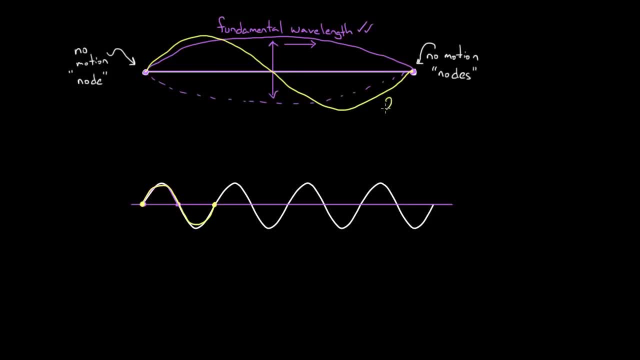 That would be the next wavelength. Sometimes this is called the second harmonic. Second because it's the second possibility, Harmonic because these are resonances, and this term is used a lot when you talk about resonances with musical instruments. What would the third harmonic look like? 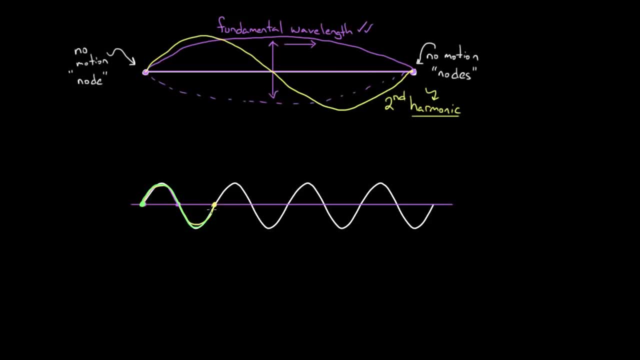 Well, we gotta start at a node. We go to this one. That was the fundamental. This is the second harmonic, So that's gonna be the third harmonic. So this one's gonna come up, It's gonna go down, It's gonna go back up. 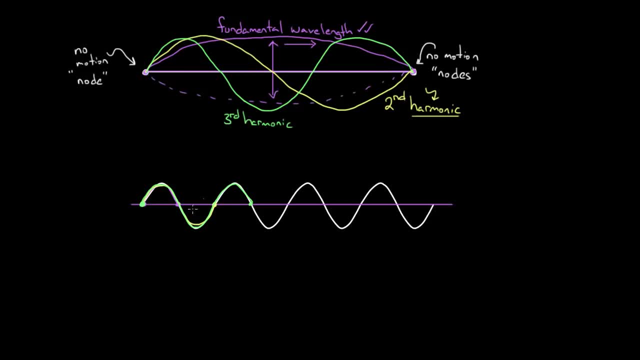 And then it's gonna come back down. That would be the third harmonic, And you can see, you can keep going here. You can create infinitely many of these, But let's analyze what's going on up here. What's actually happening in these standing waves? 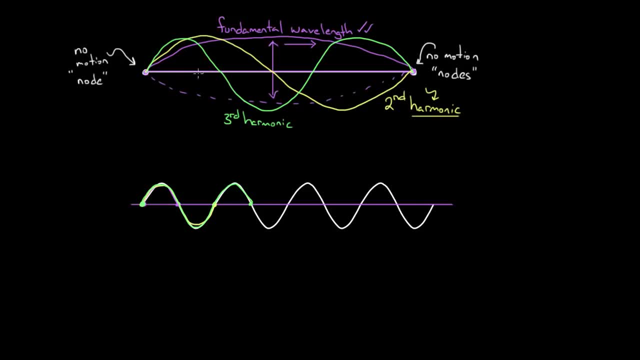 Note that there's gonna be points like right here on this third harmonic And if I draw its mirror so that I can get this. So this is what it would look like, maybe a little after, Actually exactly one half of a period after- this bold line. 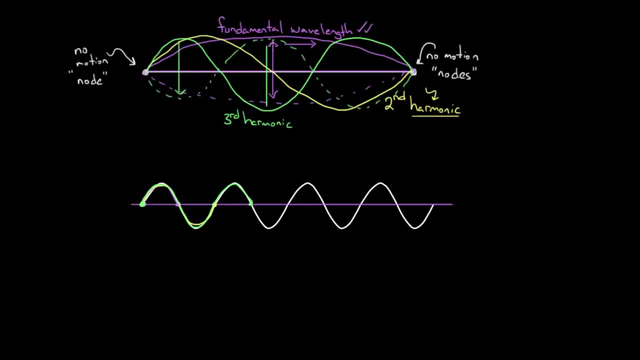 So you wait, This peak moves down to here, This valley moves up to this peak, This peak moves down here, This peak moves down to here. They're oscillating back and forth. But note this point right here, just stays put. 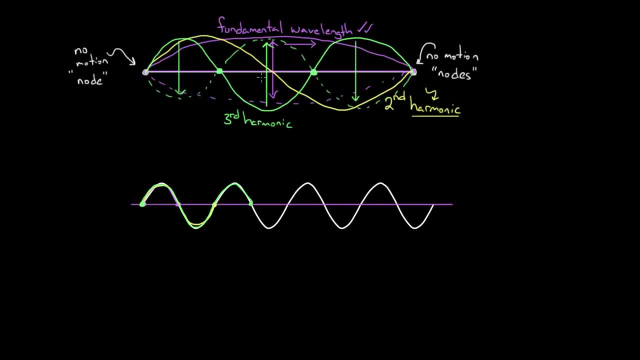 That's not even gonna move. That's a node. And so is this point right here. These points are happening because when those waves line back up, remember, the wave travels to the right, bounces back to the left, And at this point right here, and this point right here. 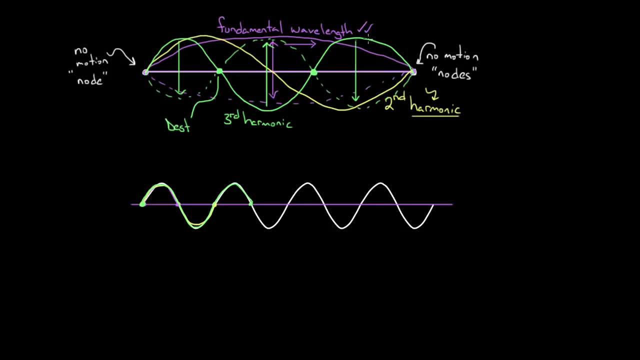 you're getting destructive interference between those two waves. Similarly, at these points where you're getting the maximum displacement, the two waves are lining up in such a way that they're interfering constructively. So the nodes are the destructive points where the wave cancels. 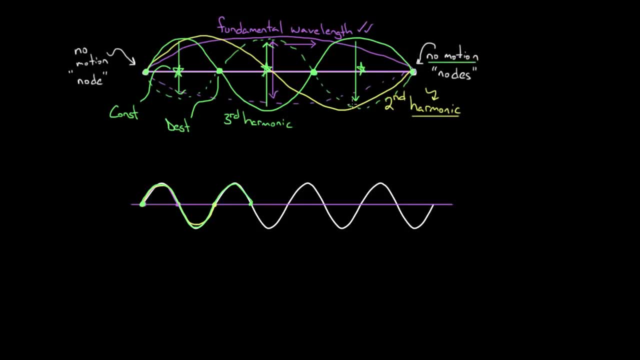 That makes sense because there's nothing happening there, There's no motion, And these maximum displacement points are the constructive points. We should give those a name. What do you think we call those? If you guessed anti-node, then you're right. 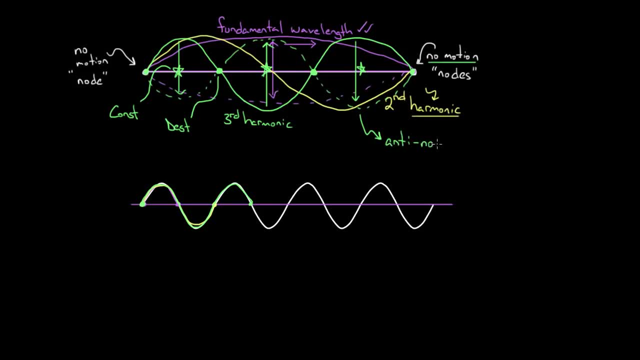 These are called anti-nodes because that's where there's the most motion. Now you often have to figure out mathematically, in terms of the length of the string, what are the actual wavelengths you can get. So drawing the picture allows you to find those. 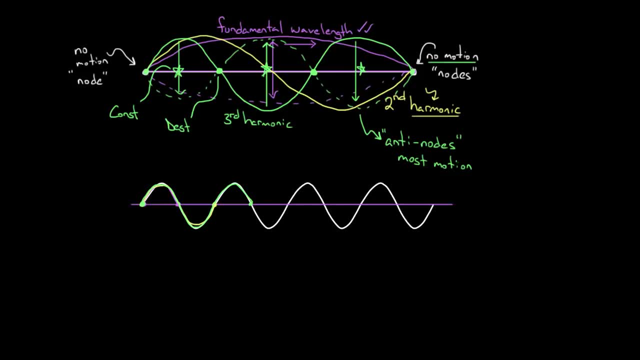 But how do you actually get them mathematically? Well, I've kind of created a horrible mess here, So let me clean this up. Sorry about that, Get rid of all that. Let me just add some strings in here, And so this doesn't get too abstract. 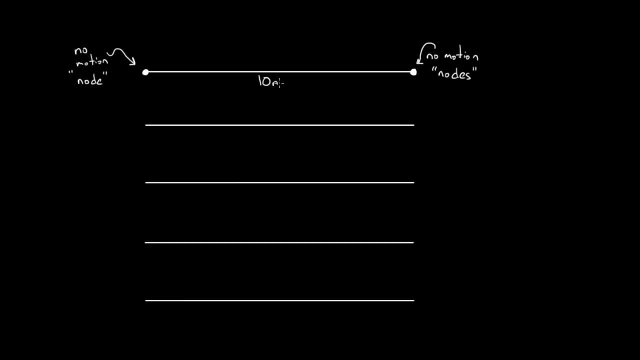 Let's just say the length of this string. it's pretty big. Let's just say it's 10 meters, A really long string you secured at both ends. So the first standing wave looked like this: Jump rope mode looked like that: 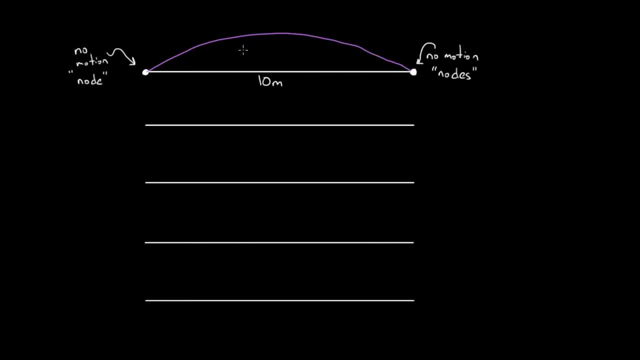 Now, if the string has a length of 10 meters, what would be the wavelength of this wave? You might say 10 meters, But no, this is not one whole wavelength. remember, If we looked at this wave pattern we had over here? 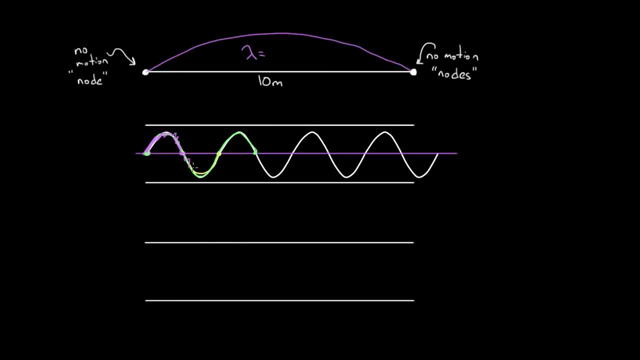 that we were using. this is one entire wavelength. You had to go all the way to here to get through a whole wavelength. This was only half of a wavelength, So this jump rope is only half of a wavelength. What would a whole wavelength look like? 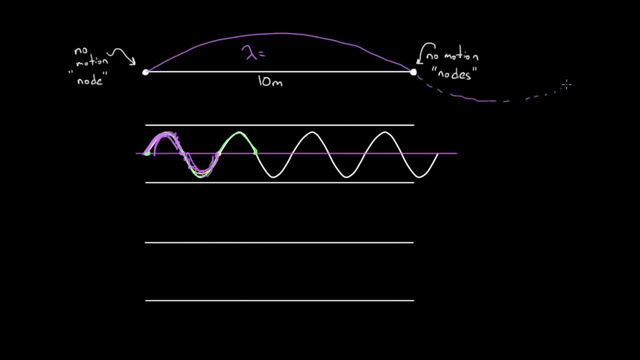 This would extend all the way out here, all the way back up. I can't really get there, so I don't go off screen. That would be a whole wavelength. So this would be 10 meters and then another 10 meters. 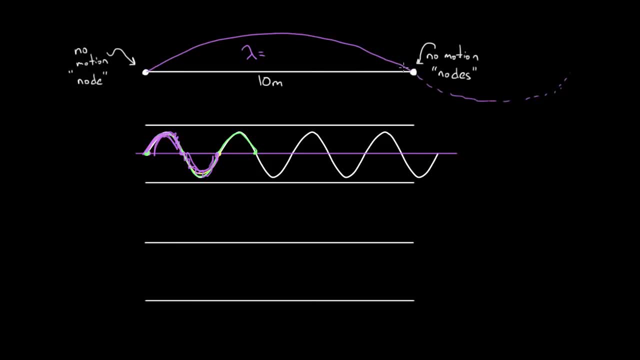 That means the wavelength of this wave, even though a whole wavelength isn't fitting in here. if there was a whole wavelength on this string, extended, this wavelength would be 20 meters. What was the next wave, Remember? it looked like this: 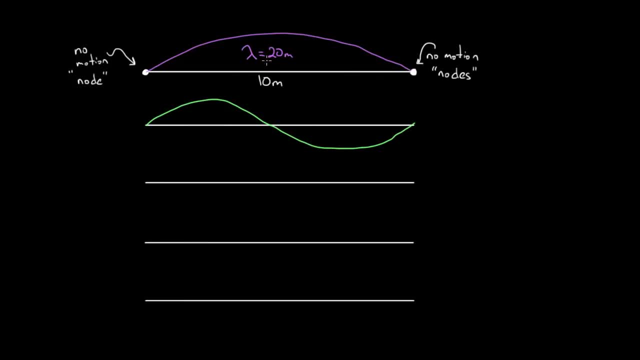 It had one node in the middle, whereas this first fundamental wavelength had no nodes in the middle. And again, if this string is 10 meters, what's this wavelength equal? Well, that's easy: This is one whole wavelength, so that would just be 10 meters. 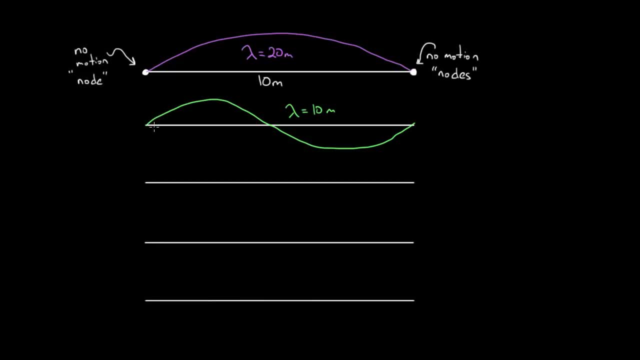 So the wavelength here would be 10 meters, because one whole wavelength fit exactly within this string's length of 10 meters. And the third harmonic looks something like this: It has two nodes in the middle. Note, you keep picking up another node in the middle. 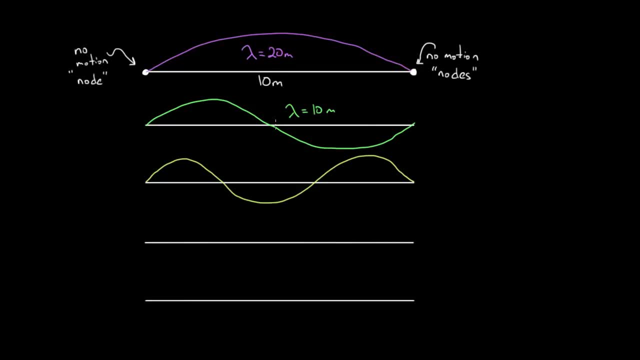 Fundamental has no nodes in the middle. Second harmonic has one node in the middle. Third harmonic will have two, The fourth will have three and so on. So what is this wavelength? This one's a lot harder for people to figure out. 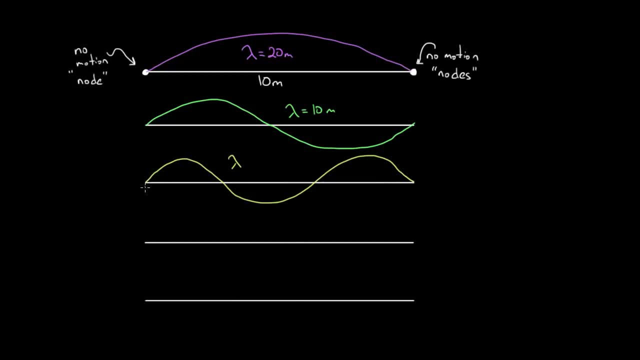 So let's look at this. One wavelength is all the way to here, So this is a wavelength, But our string is this long. So what fraction of this length is this wavelength? Well, look at it. This wavelength is 2, 3.. 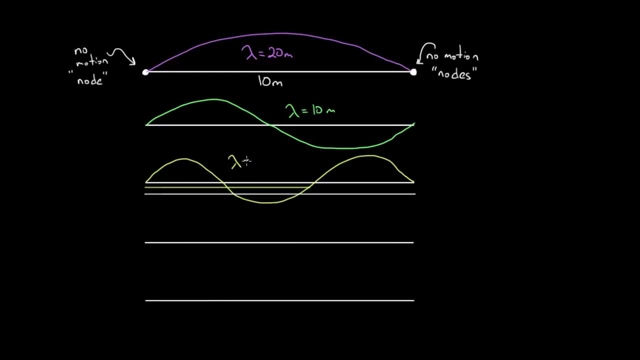 2, 3 of the entire length of the string. That means we could just say that this wavelength is 2, 3 of 10 meters, which is we could write it as 20 meters over three. And we'll keep going here. 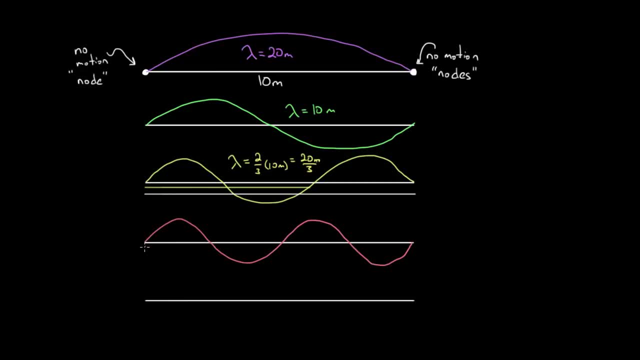 I'll draw the rest. This is the fourth harmonic. How big is this wavelength? Well, this wavelength covers half of the string. So this wavelength is gonna be half the length of the string and that's gonna be half of 10, which is five meters. 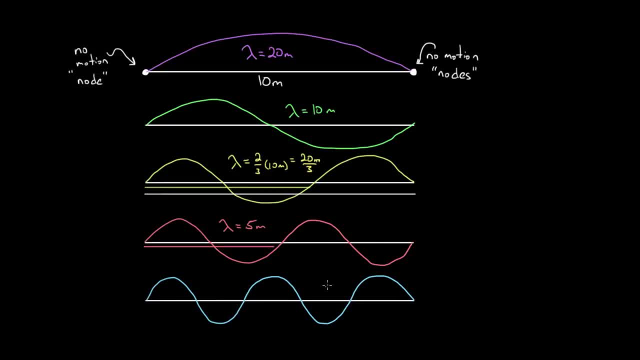 And we can keep going. I can draw the fifth harmonic down here and it would look like this: And you can ask yourself: how big is this wavelength? Well, this wavelength, let's see one, two, three, four, five. 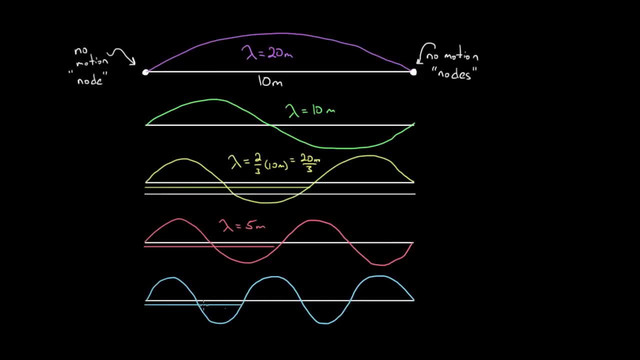 We got five of these humps in here, So this wavelength's gonna be 2 5ths of this entire length. So I'm just gonna write: lambda is two times 10 would be 20 meters. So 2 5ths of 10 would be 20 meters over five. 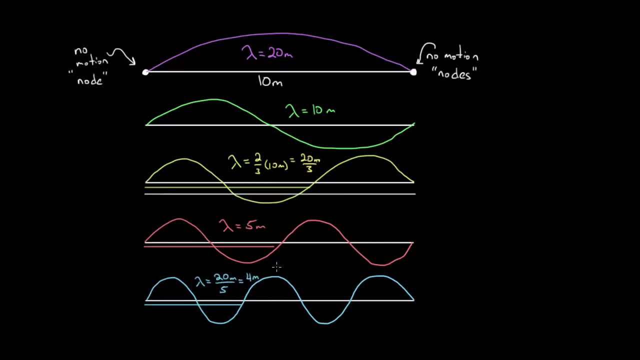 Oh, which we could simplify as four meters. But what if they asked you for like the 43rd harmonic? If they were like, hey, what's the wavelength of the 43rd harmonic? I don't wanna sit down and draw like 43 of these things. 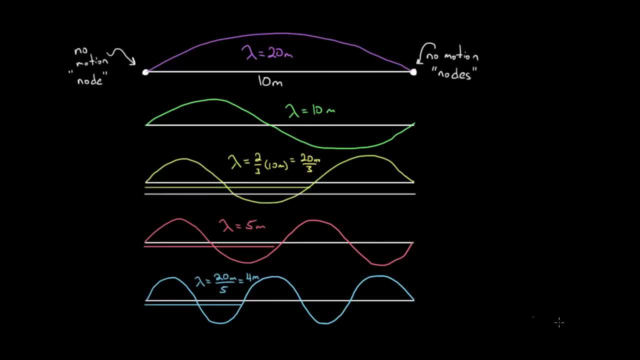 and try to figure out what fraction it is, And you don't have to. There's a pattern here, So let me show you the pattern. So this is gonna look kind of weird, but I'm gonna write this first fundamental wavelength as two times 10 meters over one. 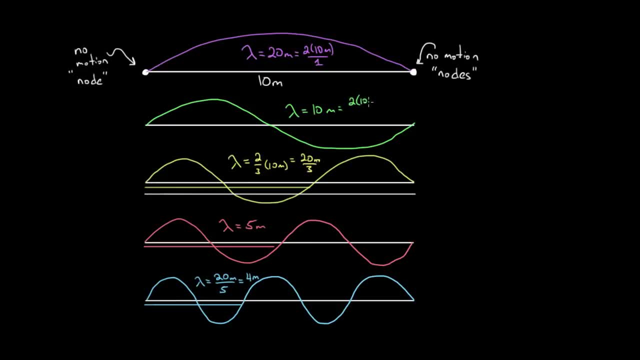 And then I'm gonna write this second harmonic as two times 10 meters over two, And I'll write this third harmonic as two times 10 meters over three. This fourth harmonic is gonna be two times 10 meters over four. This fifth harmonic could be written equivalently. 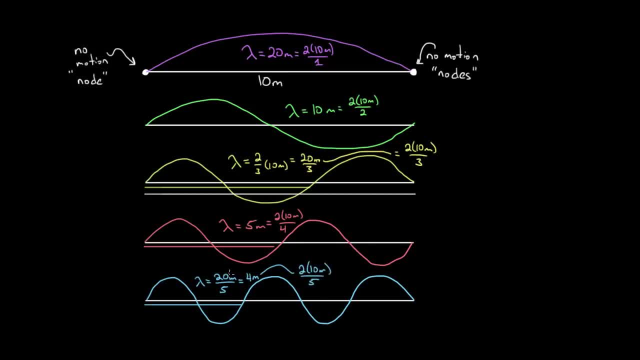 as two times 10 meters over five, since that's 20 fifths. And now hopefully, you see the pattern, You realize. okay, I see what's going on here. If I want, the wavelength of the nth harmonic n could be like the first, the second, the third. 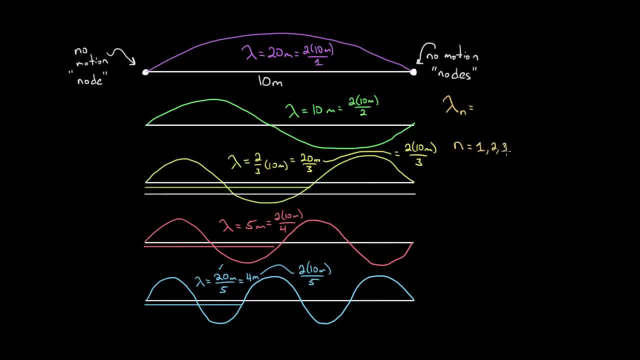 So n is really just an integer: one, two, three and so on. I can figure out what that wavelength would be simply by taking two times the length of the string. I'm gonna write it as L, So this applies to any string of any length. 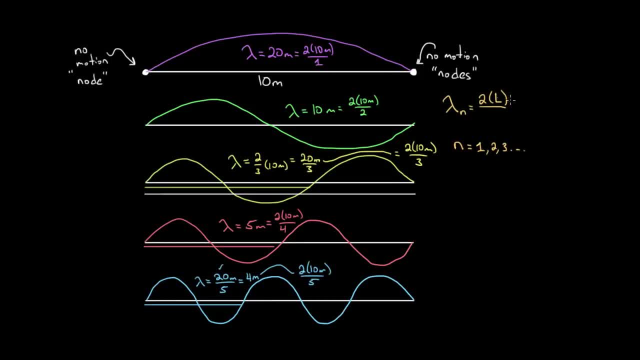 as long as it's got nodes at the end points. So take two times L and then just divide by n. So in other words, if I want the wavelength of this 84th harmonic, I'll just take two times the length of my string and divide by 84.. 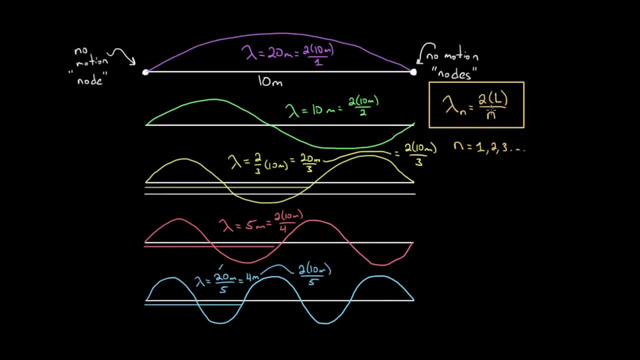 If I wanted the 33rd harmonic, I'd take two times the length of the string over 33, and that would give me the wavelength of that harmonic. Now you should remember when we derived this equation. we drew these pictures and these pictures all assume